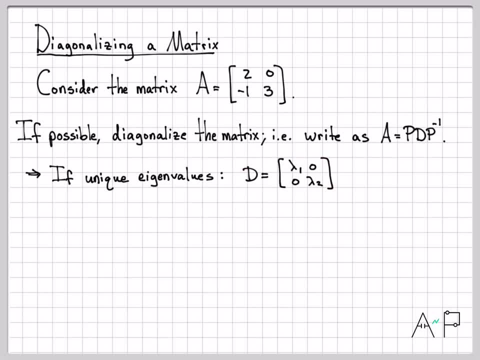 then we can construct a D by making the eigenvalues the diagonal entries of that matrix, and then the matrix P consists of the eigenvectors associated with those eigenvalues. So any matrix that you have, if it has unique eigenvalues, you can always write in this framework And 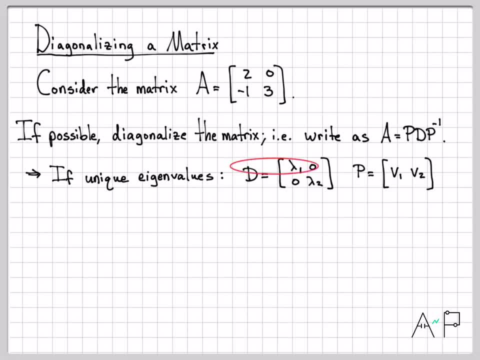 these equations right here tell us how to construct those matrices. D is always a diagonal matrix whose elements are the eigenvalues along the diagonal, and P is a matrix whose columns are the eigenvectors. So really, what we need to do is we need to figure out what 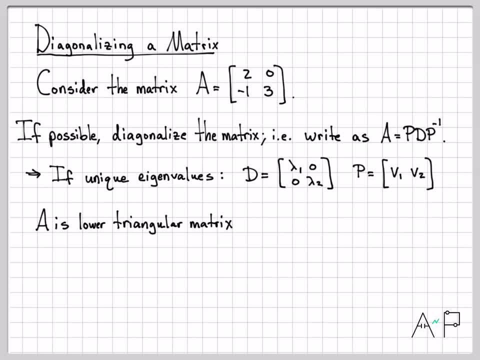 the eigenvalues and eigenvectors are of A. Note that A is a lower triangular matrix. All of the non-zero values are on or below the diagonal. That means the eigenvalues are just the diagonal entries. That means lambda 1 is 2 and lambda 2 is 3.. So we know what the diagonal elements are for our D matrix. 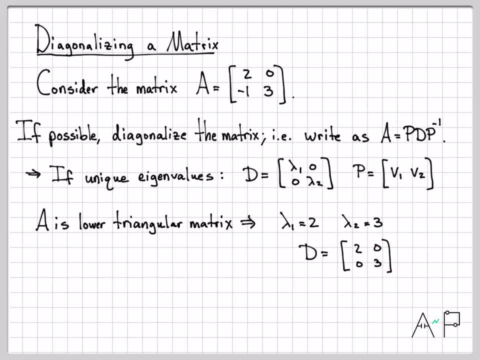 now We know that D should be this 2 by 2 matrix right here. All right, that part's done. What do we need to do now? We need to find the eigenvectors v1 and v2.. So on the 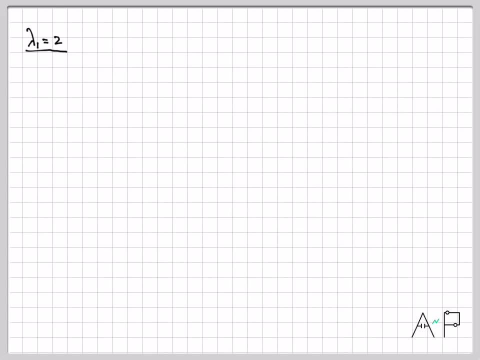 next chart we'll actually work through those eigenvector computations. All right, Eigenvalue lambda 1 is 2.. I need to find the solutions to this equation. This is what it means to be an eigenvector. So if we plug that in, we get 2 times 2, 0, negative 1, 3.. That's. 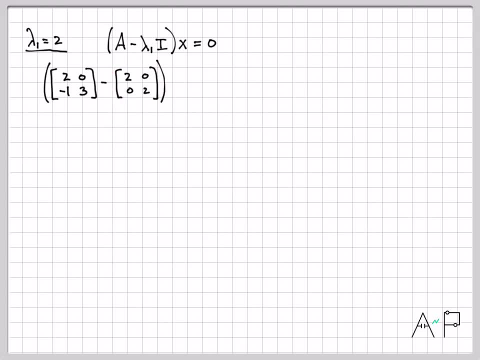 our matrix A And we need to subtract off 2 times the identity matrix because I'm working with the eigenvalue 2. And I need to find all solutions to this system of equations. So I need to find all x1 and x2 that solve this. If we simplify this just a little bit. 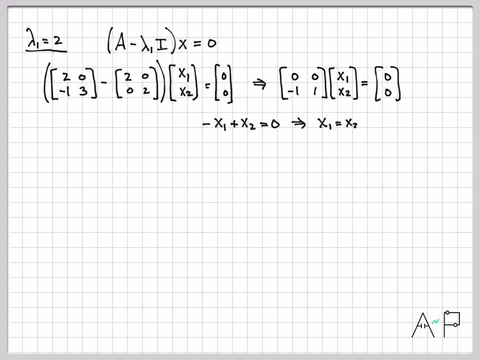 we end up with this. And if I look at that second set equation right here, this equation says that minus x1 plus x2 is equal to 0, which, if I rearrange, says that x1 equals x2.. And remember, this always happens when we do eigenvector computations. You always 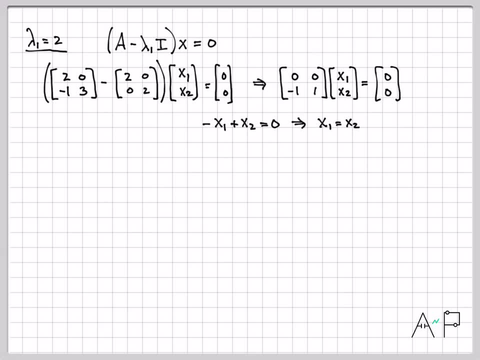 end up with free variables and an infinite number of solutions. Any solution that has x1 and x2 will be an eigenvector, So I'm going to set x1 equal to 1, just for simplicity. And since x1 is 1, x2 has to be.